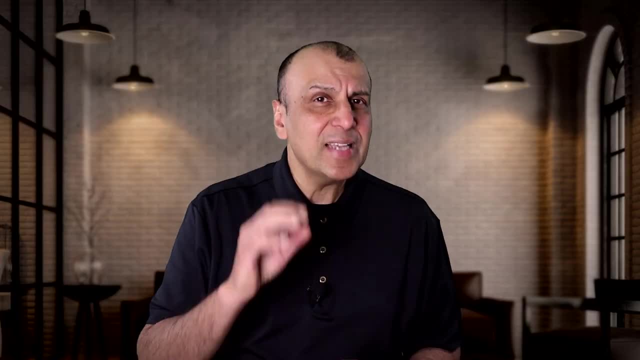 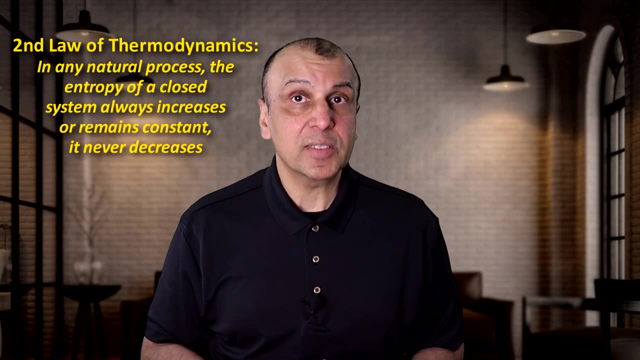 according to this equation To Stephen Hawking and others, this idea that the surface area staying the same or increasing looked very similar to the second law of thermodynamics. The second law of thermodynamics states that in any natural process, the entropy of a closed 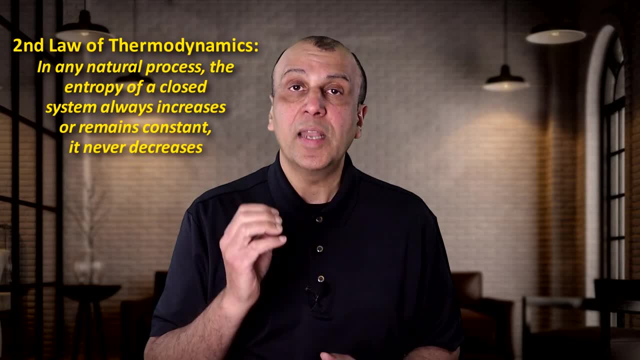 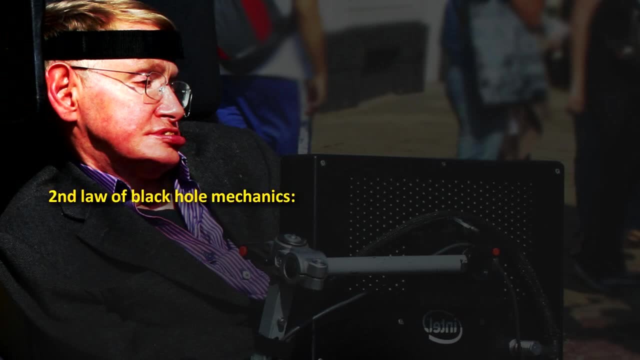 system always increases or remains constant, It never decreases. So Hawking postulated an analogous theorem for black holes and it is called the second law of black hole mechanics And it says: in any natural process, the surface area of the event horizon of a black hole always. 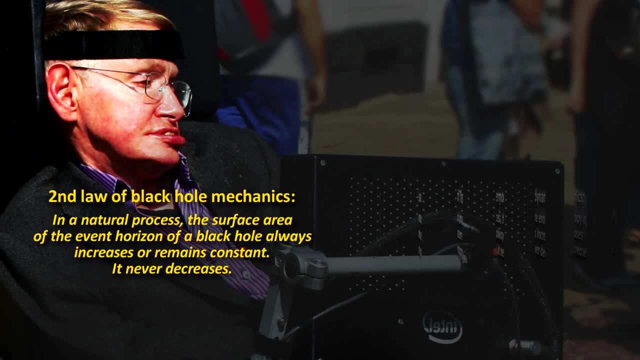 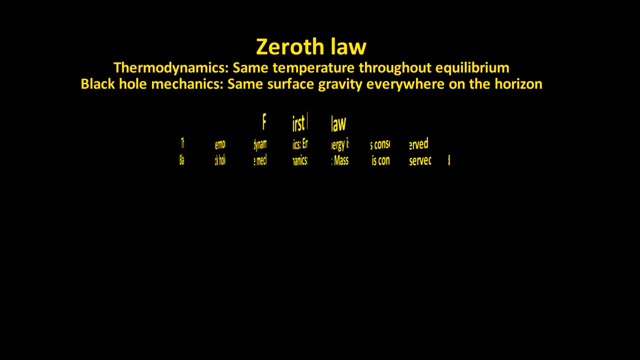 increases or remains constant. It never decreases. So now you can see the parallels with the second law of thermodynamics regarding entropy, And similar to the second law, there are also ways to state the other three laws of thermodynamics in a way that are true for black holes as well. 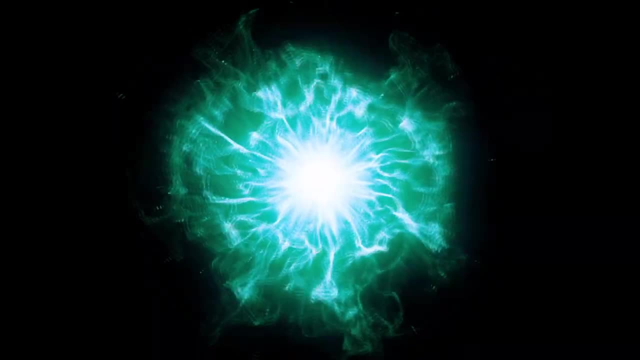 The analogy with the law of thermodynamics is that the second law of thermodynamics is the law of thermodynamics. The theory with the laws of thermodynamics suggests that perhaps black holes are physically a thermal body. In thermodynamics there is something called a. 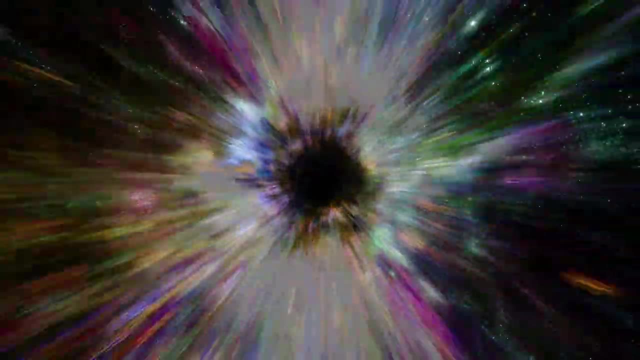 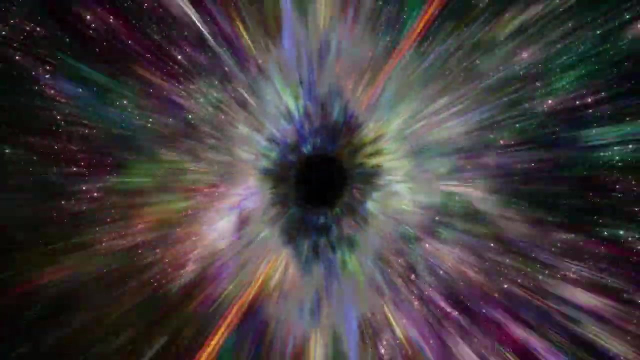 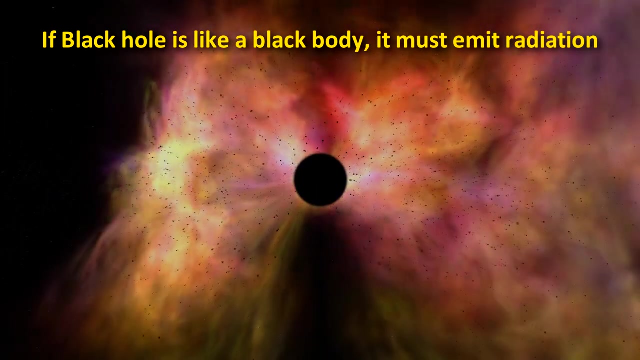 black body. A black body is something that doesn't transmit or reflect any radiation. It only absorbs radiation. So, analogously, a black hole is something that also doesn't transmit or reflect any radiation. It only absorbs it. If a black hole can be thought of as a black body from 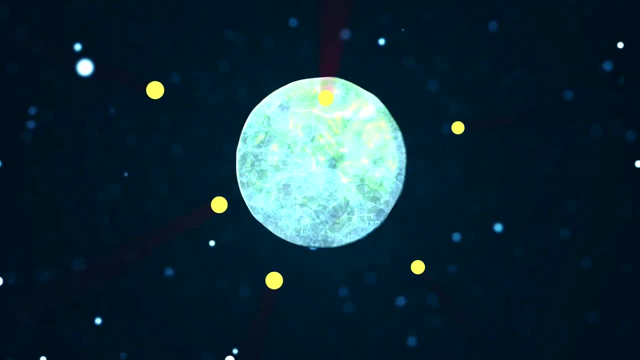 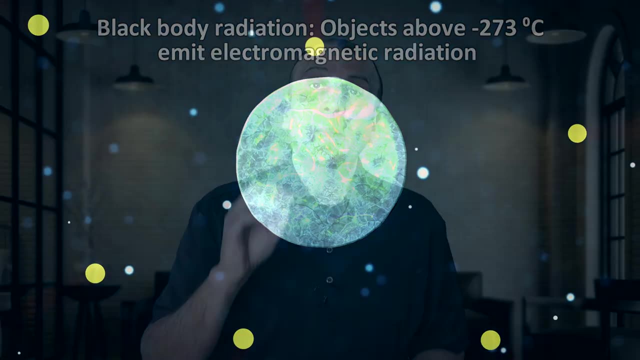 thermodynamics, then it must have a temperature associated with it, Because a black body in thermodynamics always has a temperature. But if it has a temperature it must shine in some way. But now we have a conundrum because according to classical 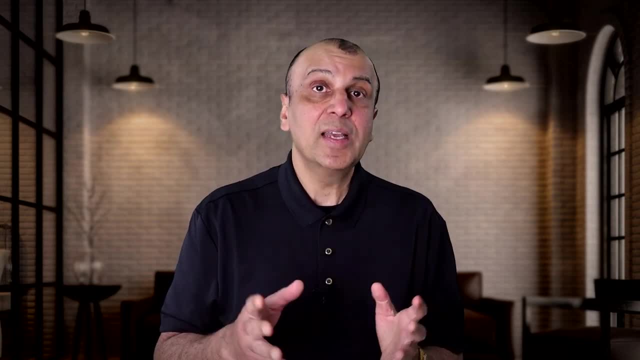 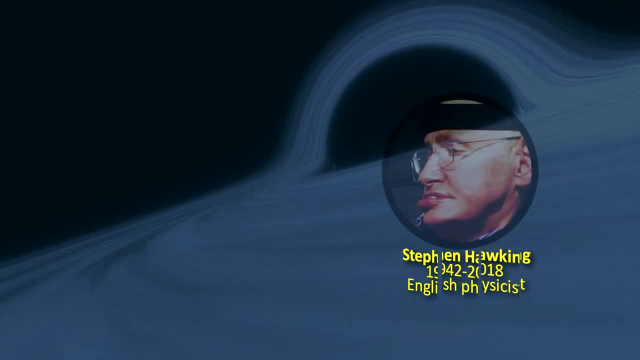 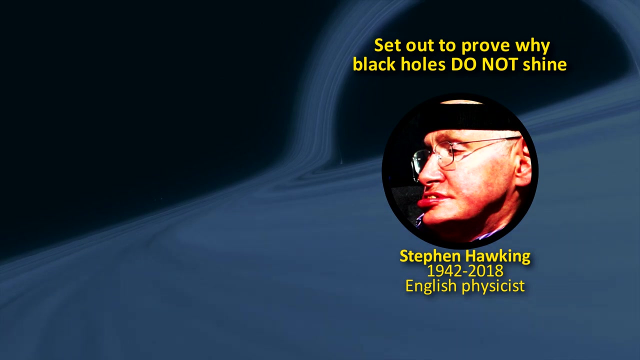 physics, a black hole is not supposed to release anything. Stuff can only go in. No stuff is supposed to come out. So how do we reconcile these two thoughts? When Stephen Hawking saw these ideas, he found the idea of shining black holes to be preposterous. He set out to prove why they would. 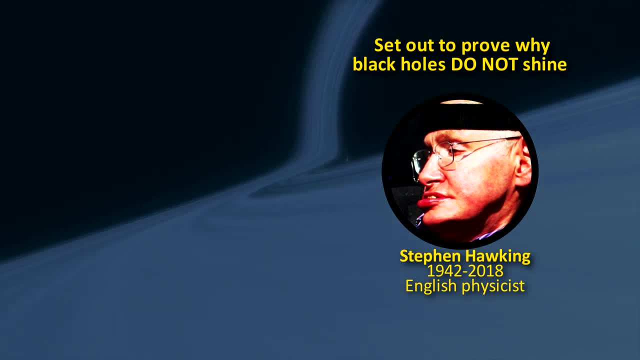 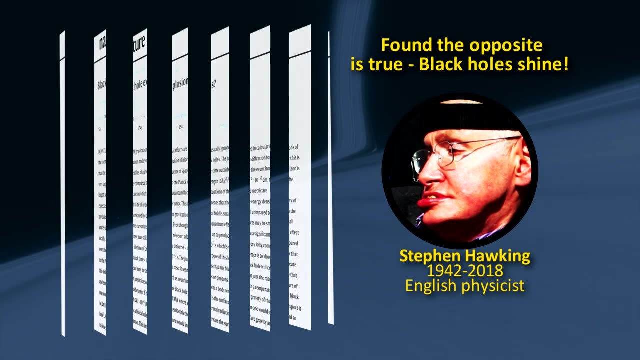 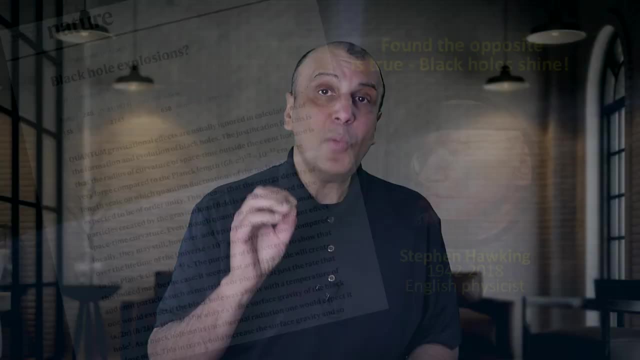 not shine. But when he applied the laws of quantum mechanics to general relativity, he found the opposite to be true. He realized that stuff can come out near the event horizon of a black hole, And in 1974, he published a paper where he outlined a mechanism for this shine. So what was the 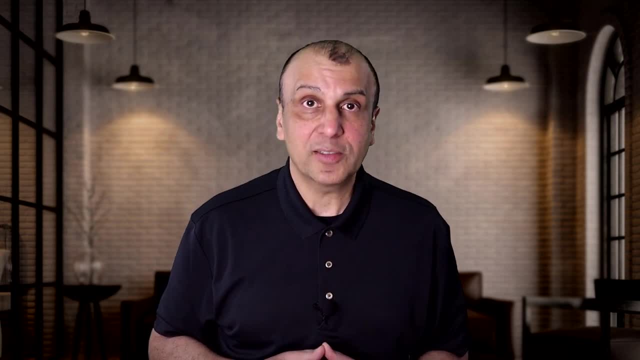 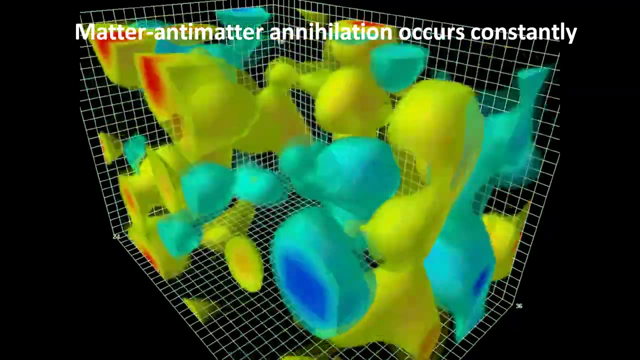 mechanism he outlined that would allow black holes to emit photons. So the simplest explanation is this: All of space is teeming with virtual particles that come in and out of existence all the time and everywhere. This is based on the Heisenberg uncertainty principle. One version of the uncertainty principle can be written as the: 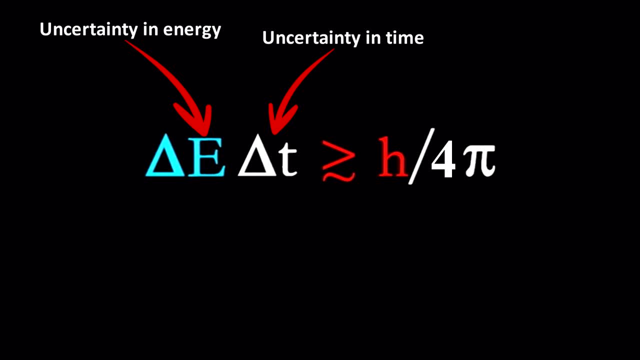 following: Delta E times delta T is greater than or equal to H, which is Planck's constant over 4 pi. So basically, what this equation says is that the uncertainty in energy and uncertainty in time are inversely proportional to each other, because the product of the two is equal to a constant. 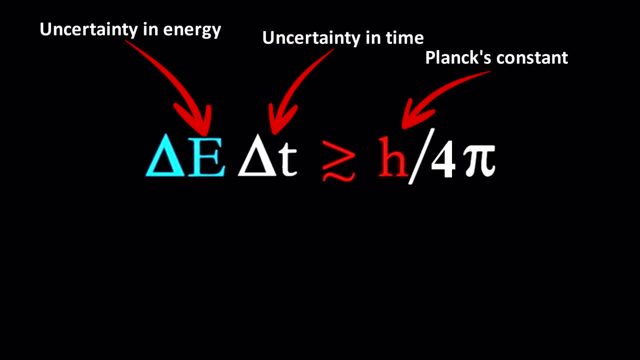 In other words, if you know very precisely the energy of a system, then you can't know the time over which you made that measurement very well. Or vice versa: You can know the time very well, but not the energy. But what this equation also tells you is that you can get. 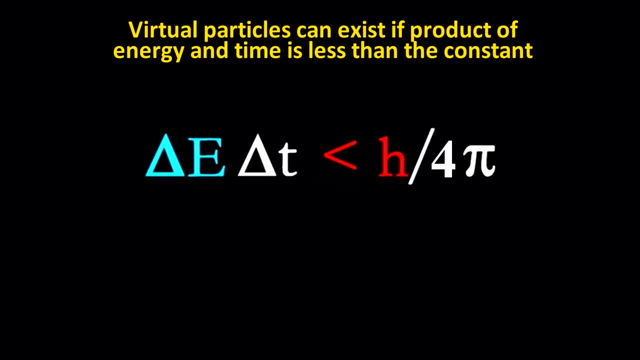 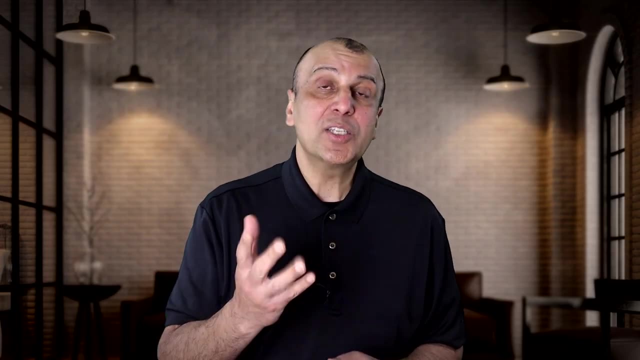 particles with an energy, delta E and, if it occurs over a very short period of time, delta T, such that the product of the two is less than Planck's constant over 4 pi. That is, particles can exist that violate this uncertainty principle. How is this possible? Well, this is one of the crazy. 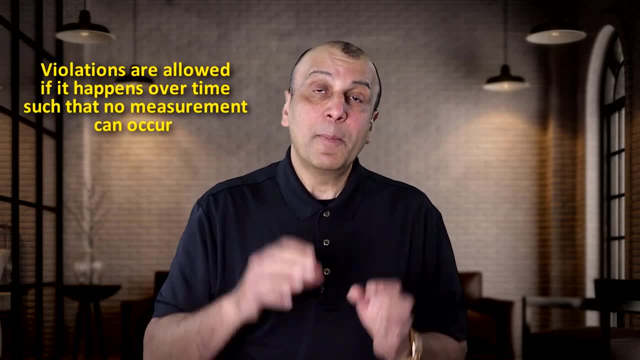 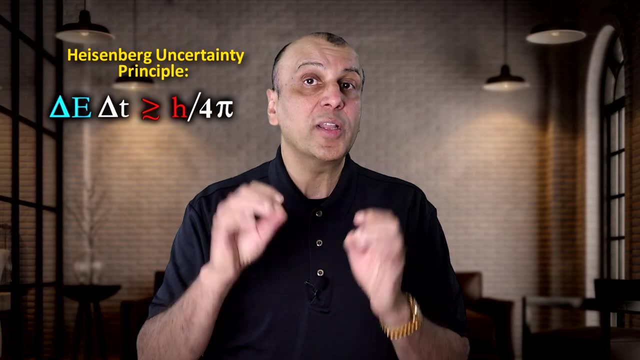 things about quantum mechanics. Violations are allowed, But it's as if, by not obeying this Heisenberg uncertainty principle, the universe really doesn't register or record its existence, because no measuring device would ever be able to measure this directly. A particle with some 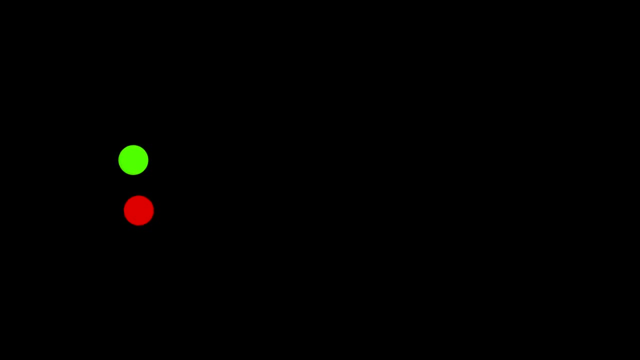 finite energy, as long as the change in time is very small, can exist. So what's happening is particle-antiparticle pairs borrow energy from the present and give it right back in the future by annihilating themselves. This is how virtual particles are formed in empty space, and space is. 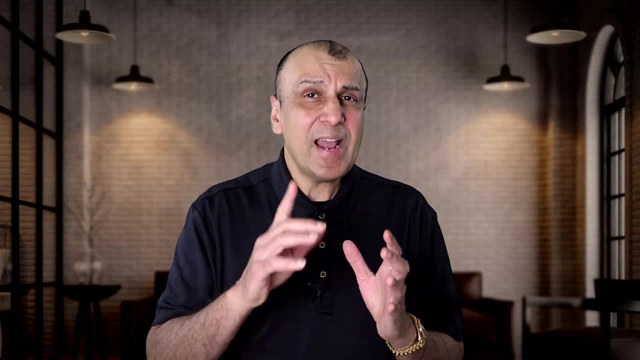 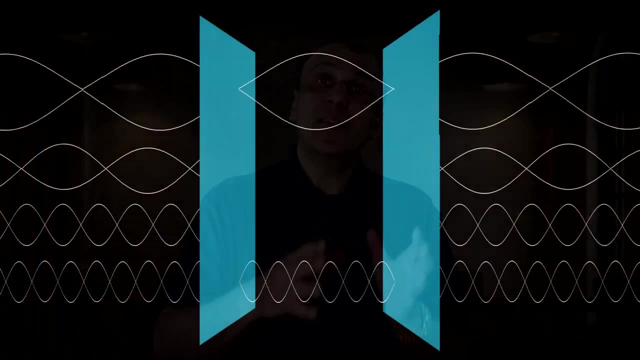 teeming with them. This is also called the question Quantum Foam. You might ask: if we can't measure it, how the heck do we know that it actually is happening? Well, it does affect the universe in ways that are measurable. For example, it manifests. 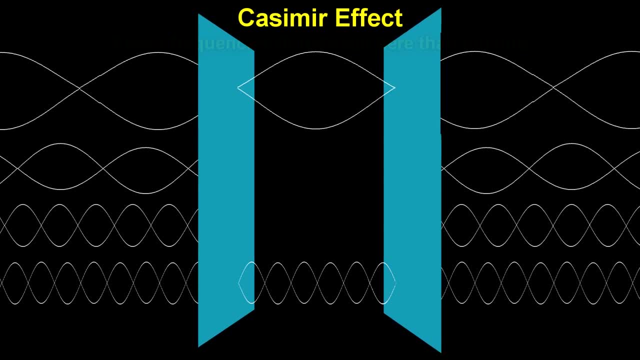 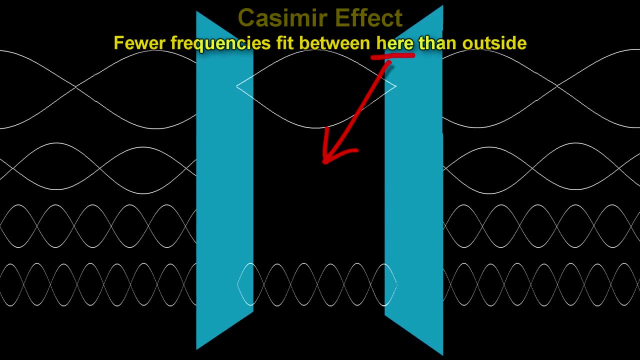 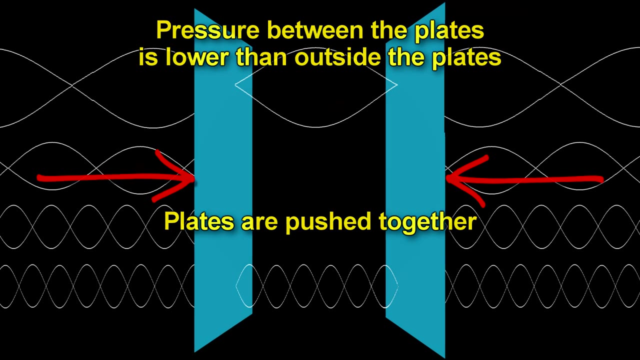 as a force in something called the Casimir effect, in which the quantum foam outside a set of two plates is greater than the pressure inside the plates and this creates a force pushing the plates together. So this virtual particle creation annihilation does really exist and is a central part of quantum mechanics. 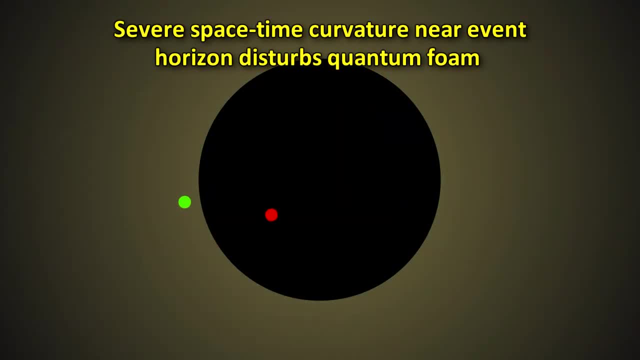 The Severe Curvature of Space. The Severe Curvature of Space time near the event horizon of a black hole disturbs this quantum foam in ways that you don't see in normal empty space, As neutrinos and antineutrinos, and electrons and positrons and other particle-antiparticle pairs get created, sometimes when two of these 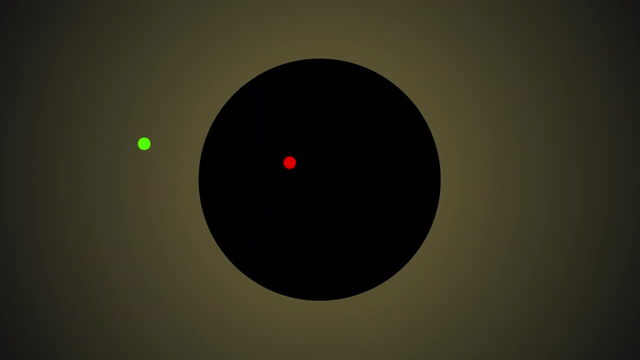 particles are close to the event horizon. one particle can get sucked into the black hole before the two particles have a chance to annihilate each other. This kind of capture and release by the black hole can happen anywhere in the space around the event horizon. 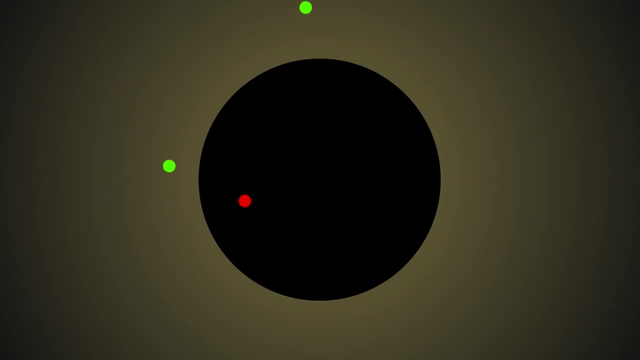 So you obvious do not understand that the World can turn black quartz 198° in In the ikos처럼 map. If the partner is left outside, it will no longer have a partner with which to annihilate, So it will remain an the escape from the black hole And this particle will be carrying energy. 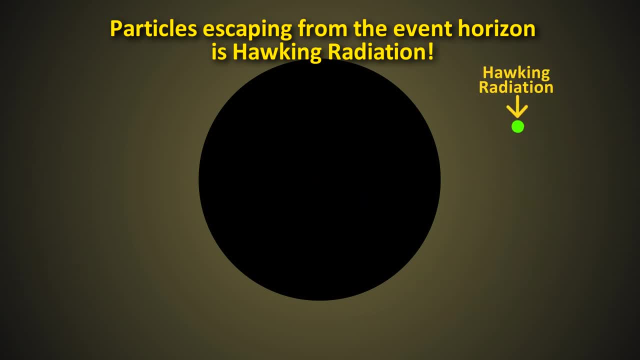 with it. this is what is perceived as Hawking radiation, And this is how the black hole shines. Where does this energy of the escape particle come from? From our perception outside than black hole, the particle we got is positive, but this means it was the black hole with no energy itself. 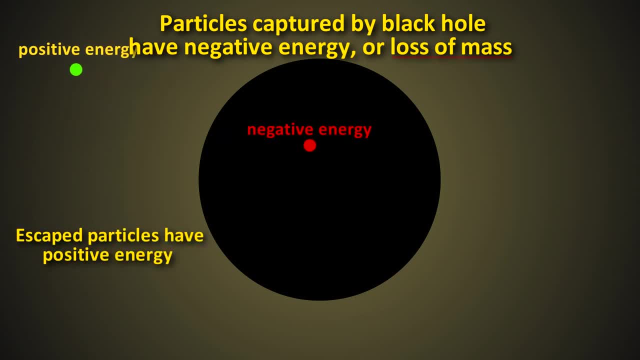 That means black hole no longer has energy. The black hole simply doesn't last particle which has negative energy. In other words, the black hole lost energy. This is the same thing as losing mass because of the mass energy equivalence of Einstein's famous equation. 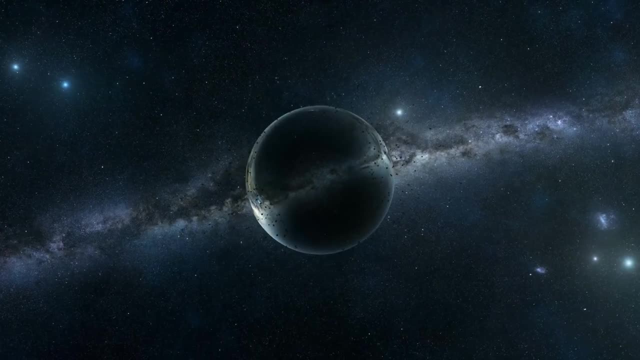 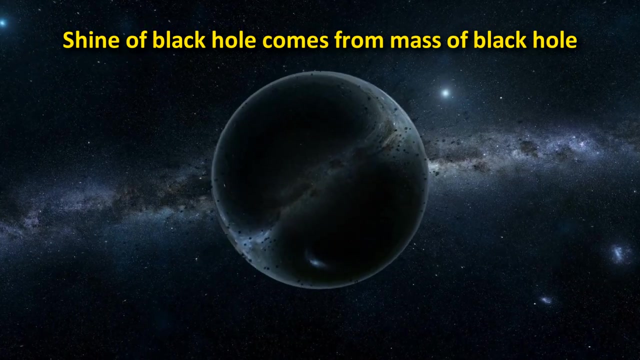 equals mc squared. So virtual particles are created in space by borrowing energy, but ultimately so that nothing violates the law of energy conservation. the energy of the shine is really coming from the mass of the black hole. So this is the popular way to think of Hawking radiation. but 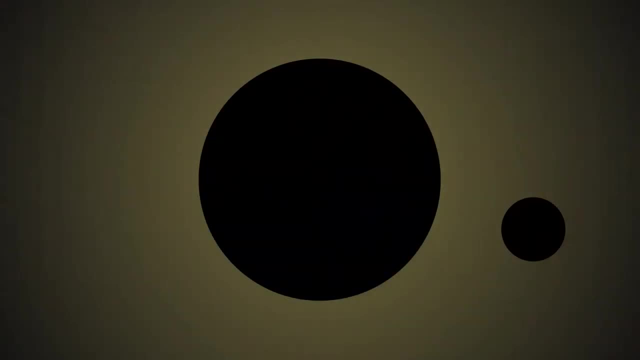 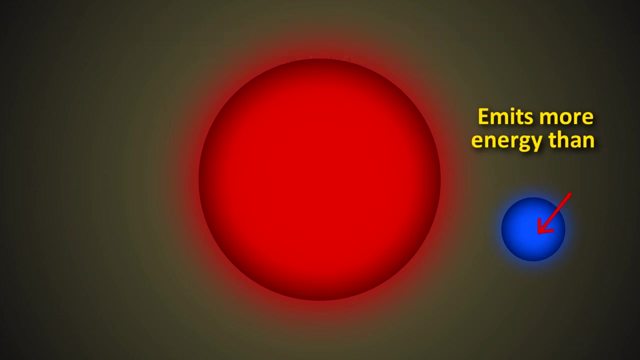 it has some problems. I think the biggest problem with this is that the radiation from the black holes is not in all different wavelengths as would be expected. with this mechanism, The radiation actually has a wavelength equal to about the size of the black hole, So smaller black holes emit shorter wavelengths or more energy than larger black holes. 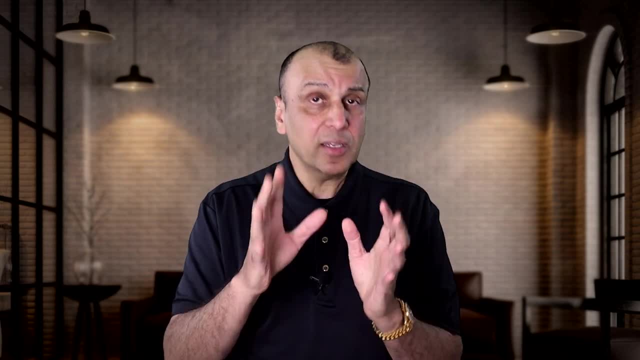 So a more accurate way to look at this is the following: Now, this is still an approximation, but it's probably a closer approximation. In reality, there are no particles, only fields. And this is the question: How do we know that there are no particles? 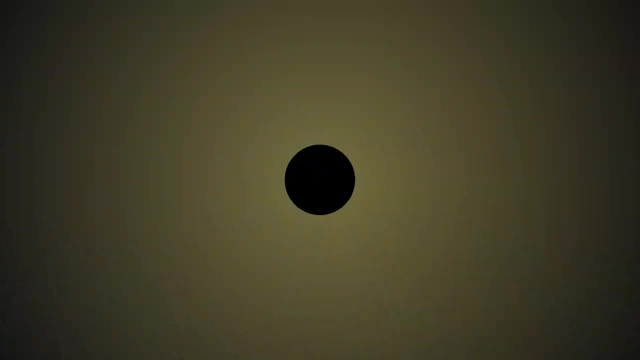 This is the crux of the quantum field theory. The actual Hawking calculations consider the waves coming in from infinity and being scattered or disrupted because of the black hole event horizon as it was forming. Certain vibrations of waves are deflected by the gravitational field of the black 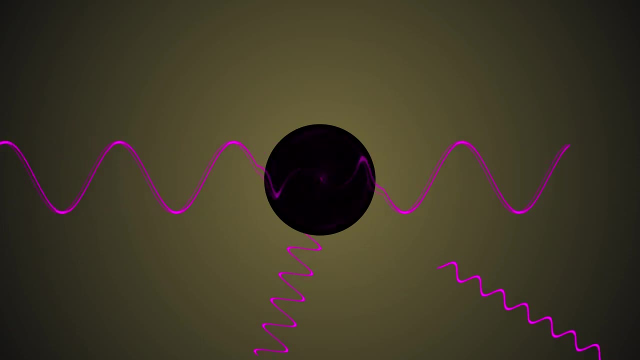 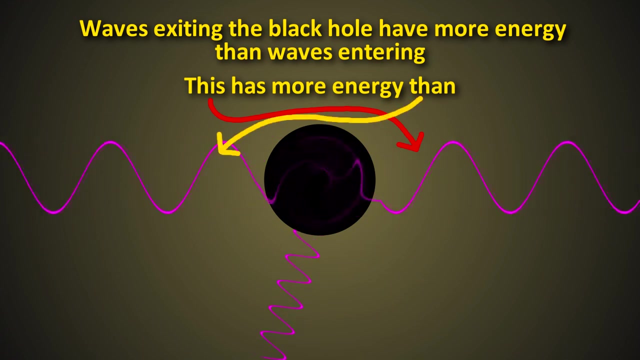 hole as it forms in the past. Some of these get distorted or even absorbed by the event horizon. Some waves don't get deflected at all. Hawking showed that the waves entering the event horizon was disrupted in a way that the wave on the other side carried away energies corresponding. 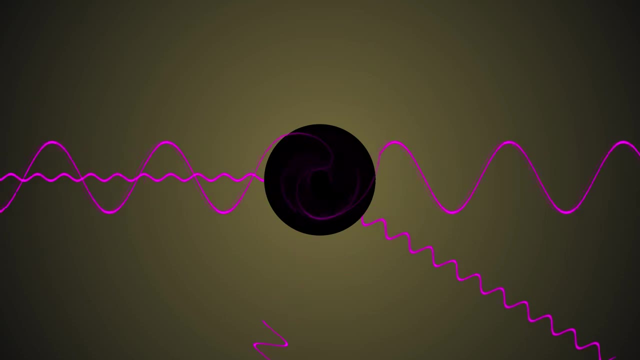 to the size of the black hole. Particles with waves as large as the event horizon get lost within the event horizon. So the energy we see are about as large as the event horizon. The quantum fields that have wavelengths the size of the black hole get out with more energy than 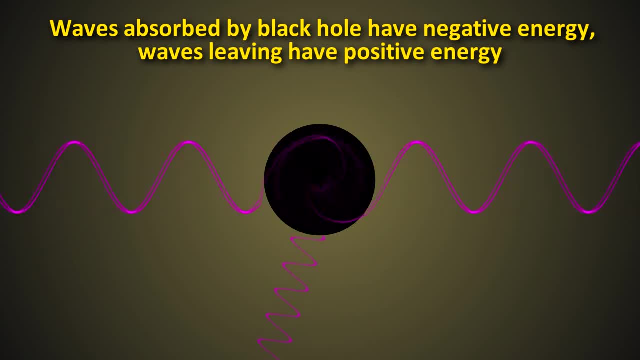 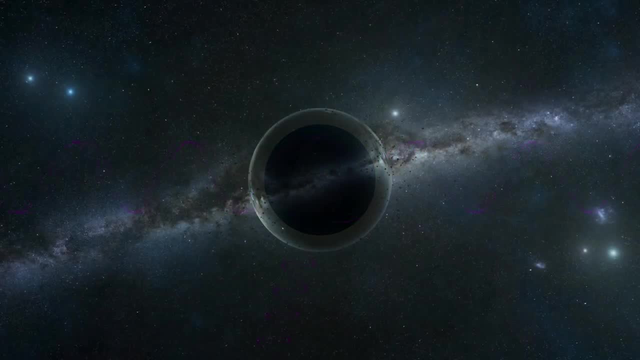 they came in with, Because waves that get absorbed by the black hole have to be negative energy in order for us to see the positive energy in our universe. This corresponds to an energy spectrum analogous to a black body at a certain temperature. So this is why black 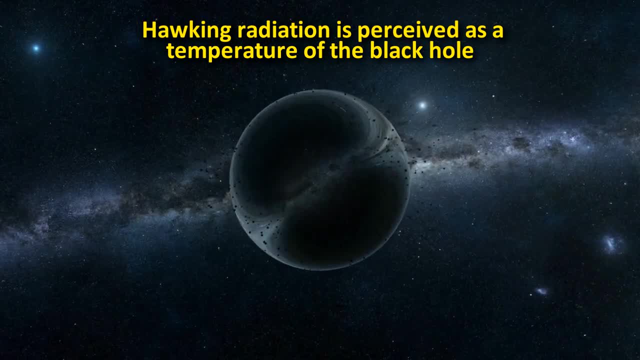 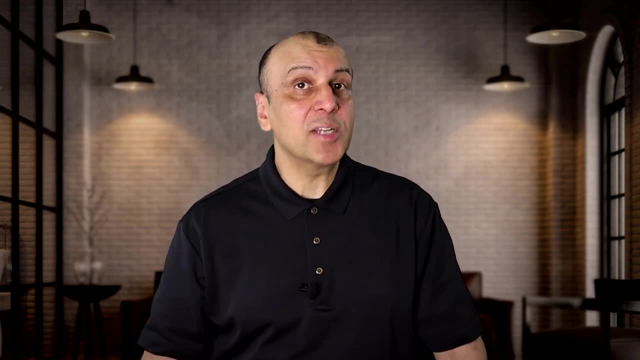 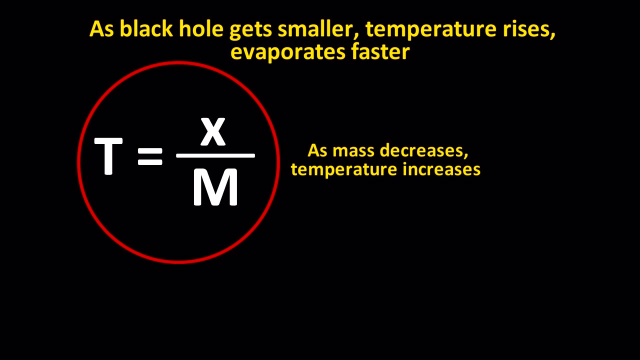 holes have a temperature and this is what we perceive as Hawking radiation. But is Hawking radiation real? Can we measure it? Not directly, but Hawking found a formula for the temperature of a black hole. Note that the temperature is proportional to the reciprocal or inverse of the mass As the black hole evaporates over time. the m in the 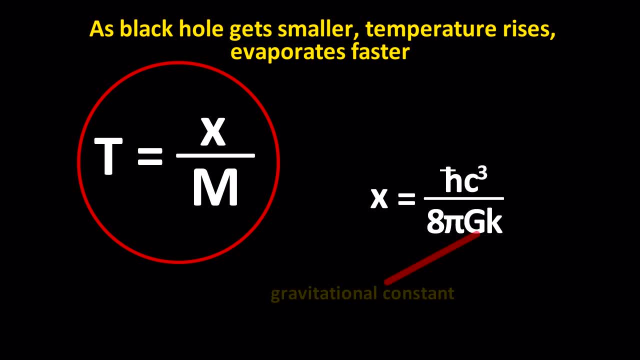 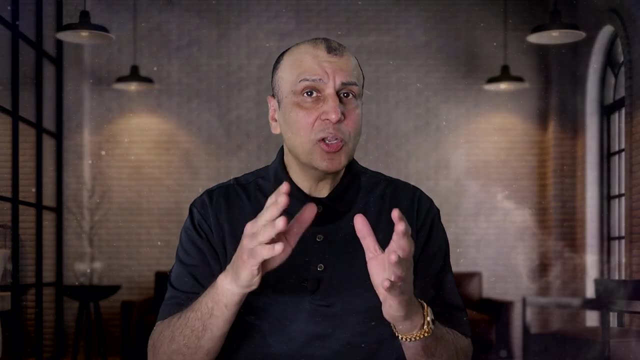 equation becomes smaller and smaller. This means that the temperature rises as the black hole evaporates. As the black hole evaporates, its mass decreases. So the hottest black holes are the smallest one. This is why they lose energy faster. Now here's the interesting part: As the mass goes, 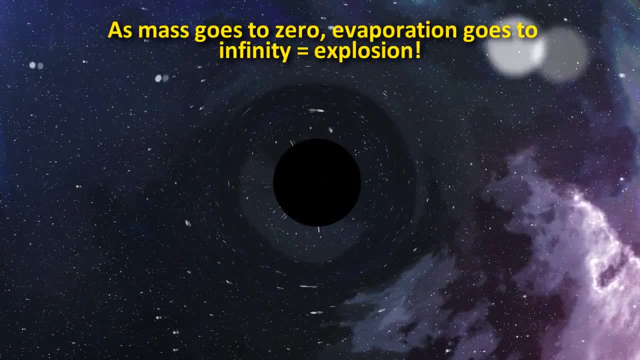 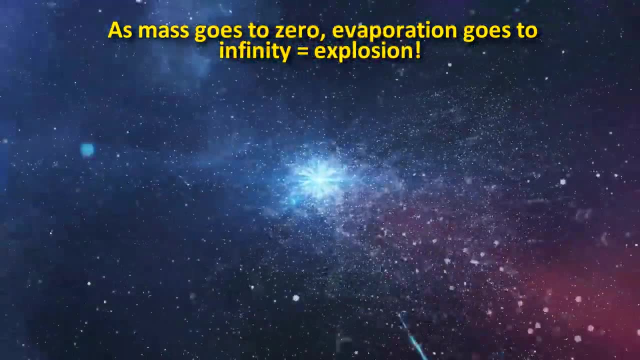 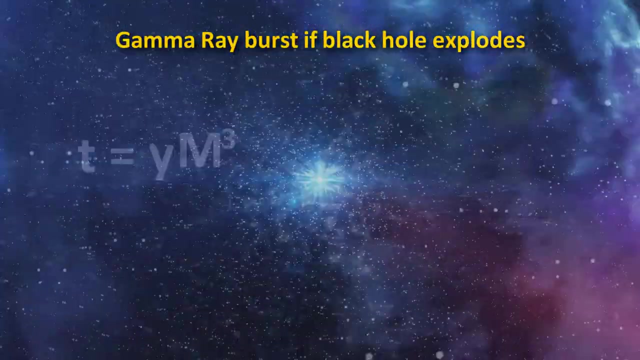 to zero. the evaporation rate goes to infinity. So this tells us that near the end of the evaporation process we would see an explosion of the black hole. as the mass is quickly used up. This would be seen as a burst of high energy photons, or gamma rays. The lifetime of the black hole is calculated. 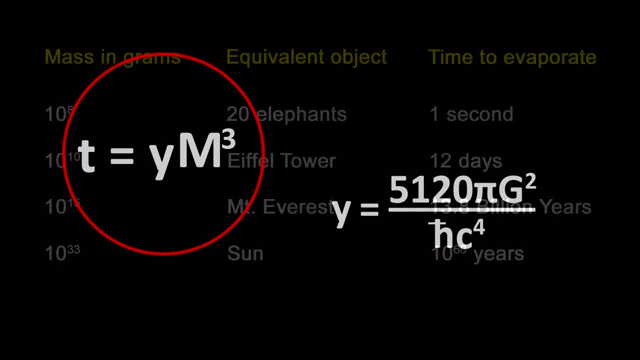 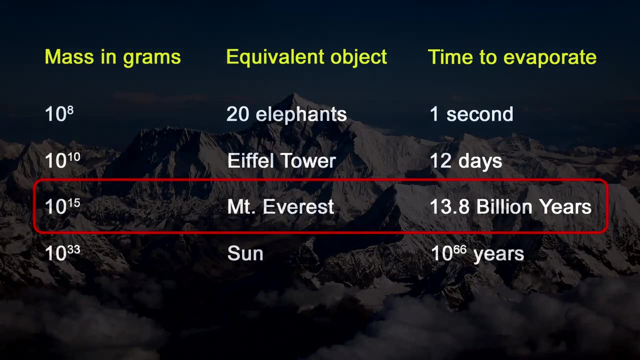 using this equation, If you do the calculations, it means that anything with a mass less than 10 to the 15 grams would have evaporated by now. This would be tiny black holes about as massive as Mount Everest. They would only be about the size of a proton, by the way. Hawking theory. 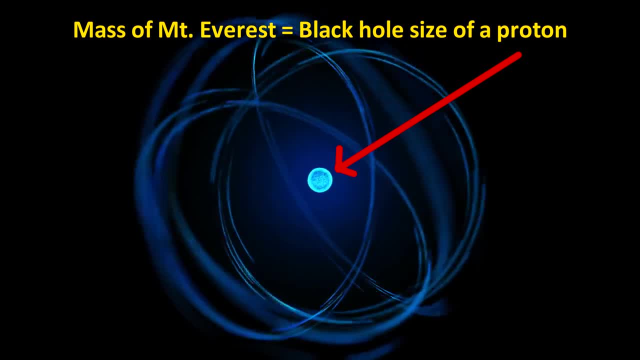 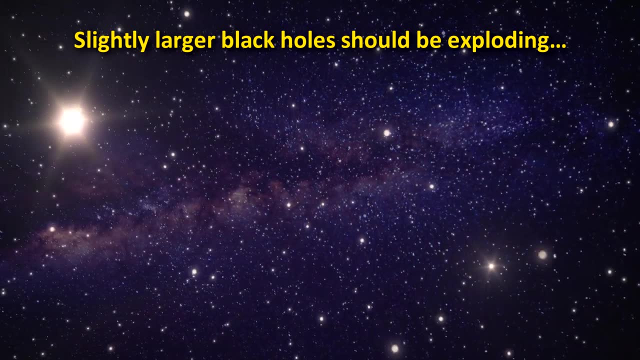 theorized that such tiny black holes could have existed at the time of the Big Bang, But it also means that black holes slightly larger than 10 to the 15 grams would be evaporating around this time in our universe, And if this is happening, it means that we should see a bunch of gamma ray. 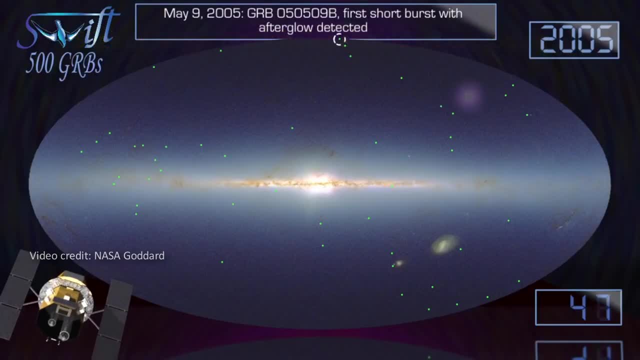 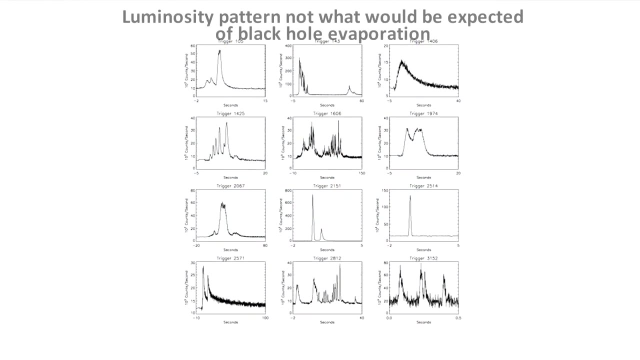 bursts. Do we detect gamma ray bursts? We do, In fact, about 1 gamma ray burst, or grv, occurs per day. However, the pattern of gamma rays don't fit with what we would expect to see in a black hole explosion. However, at a layer above deflection, it is possible that they could be used for expelling. 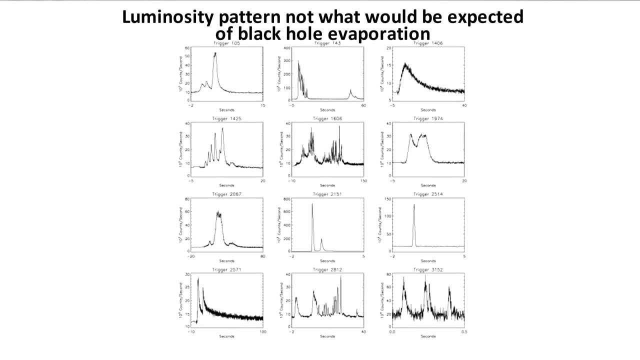 burr effect in your universe. What we see are bursts or completely blank. However, a pattern of gamma rays occurs in someHmm, by Duka ton of gamma rays which, with variations in brightness, from bright to dim to bright- again the black hole- evaporation. 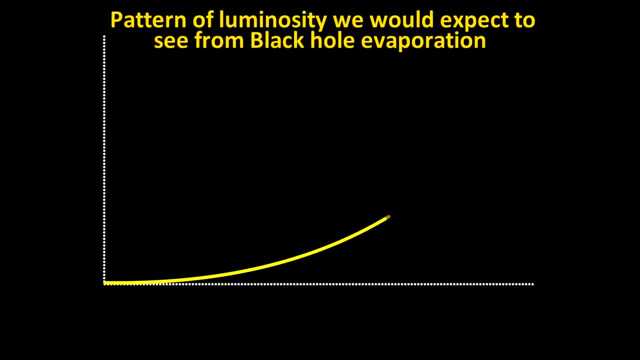 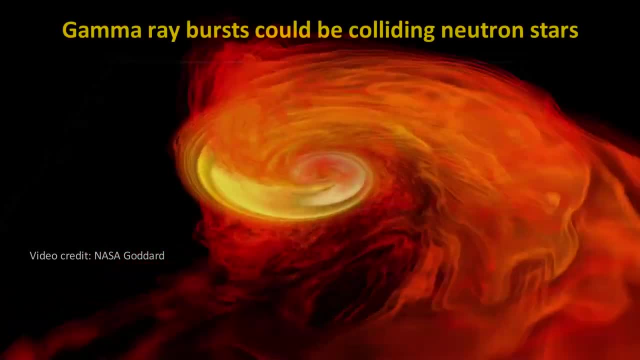 should look like a steady increase in luminosity from a low value to a high value until a final explosion. So these gamma ray bursts are attributed to another phenomenon, probably colliding neutron stars or explosions of supermassive stars, not evaporating black holes. 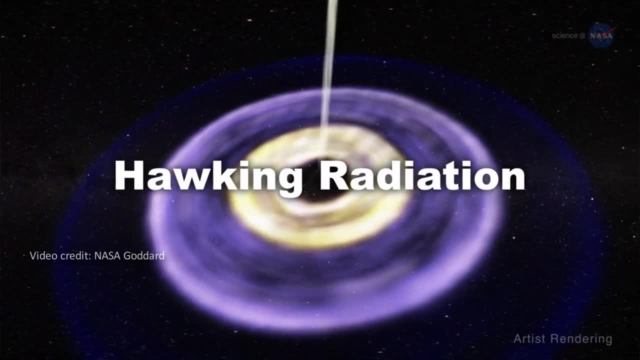 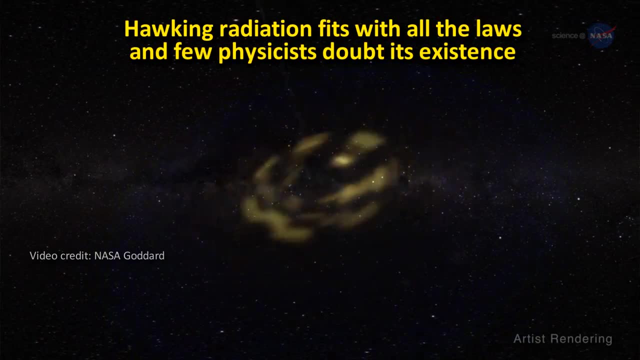 So the data doesn't really support the idea that very small black holes exist. but despite the fact that no direct evidence of Hawking radiation exists, it perfectly fits with the laws of quantum mechanics and few, if any, physicists dispute its existence. Now here's what I find incredible about black hole entropy. 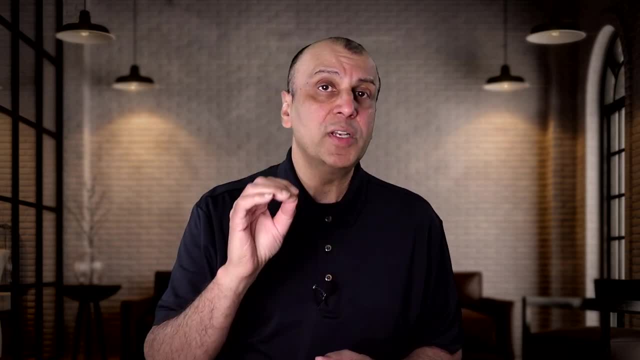 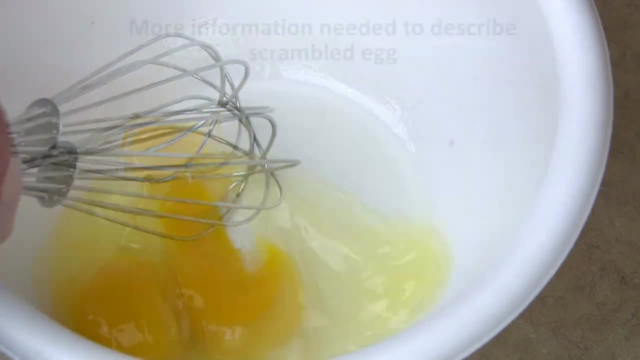 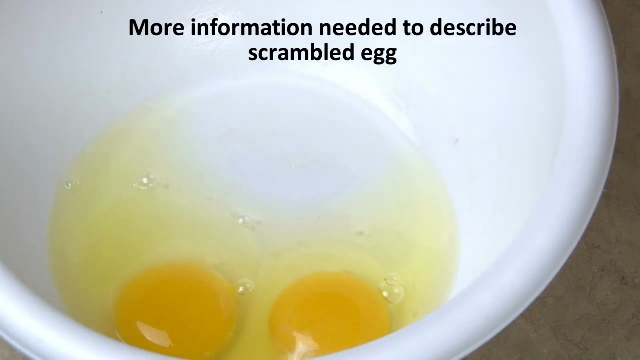 But let's clarify what entropy is. It is a measure of the amount of disorder in a system. You can scramble an egg, but you can't unscramble it. A more disordered system, like the scrambled egg, has greater entropy. You need more information to describe the scrambled or disordered state. 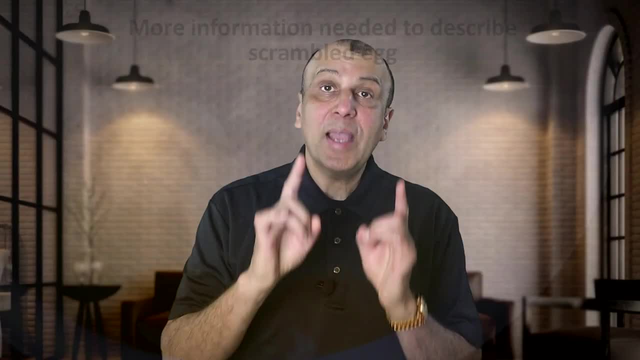 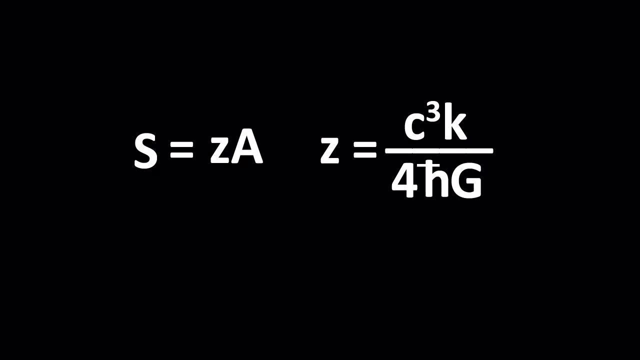 So information is also proportional to entropy. Einstein showed that the entropy of a black hole is defined by this equation: A is the area of a black hole and Z is a very large constant. This means that the entropy of black holes is a huge number. 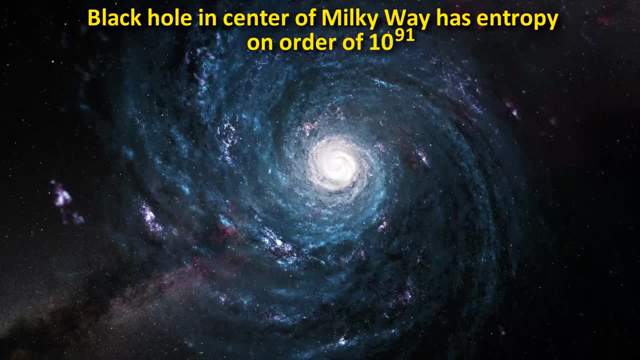 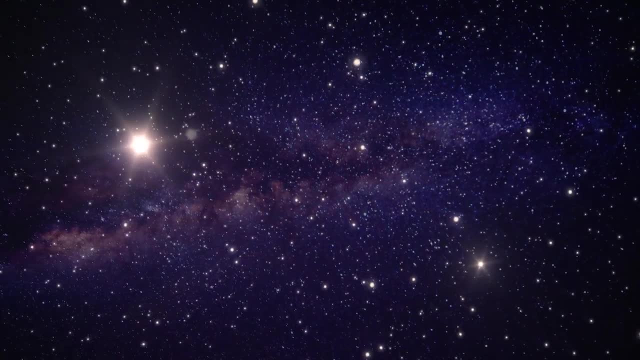 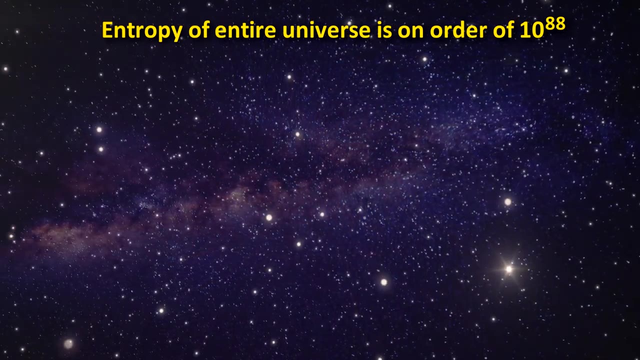 A black hole of the size of the center of our Milky Way galaxy has an entropy and the order of about 10 to the 91. Now, if you take all the entropy in the universe, ignoring gravity and other black holes, I mean take the entropy of all the matter in stars, burning fossil fuels, all the dark.